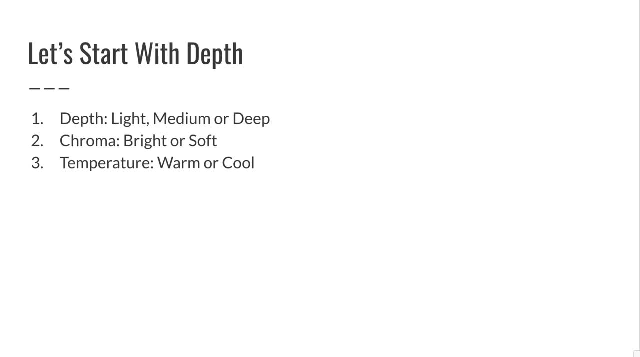 I thought I would just change things up and maybe make it a little easier for you to narrow things down. So let's start with depth. Let's go ahead and reduce the choices that you have down to four Within each category. there are four buckets of color types. There's 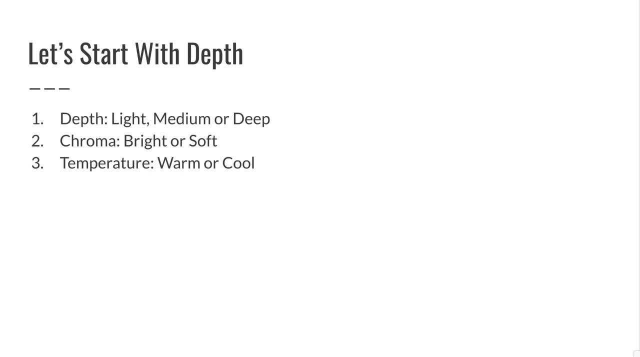 bright, warm, bright and cool, soft and warm and soft and cool, And within there you have light, medium and deep, So that's 12 total. If you can narrow it down to whether you are light, medium or deep, you've narrowed it down to just four color types And then it gets a little bit. 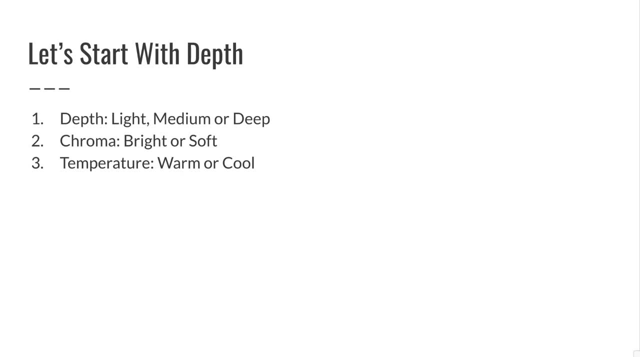 easier and less overwhelming to figure out which one of those four will be the best choice for you. Let's start with light. If you are light, you're going to have to choose the right color for you. You're going to choose your choice of red and then you're going to choose your choice of brown. 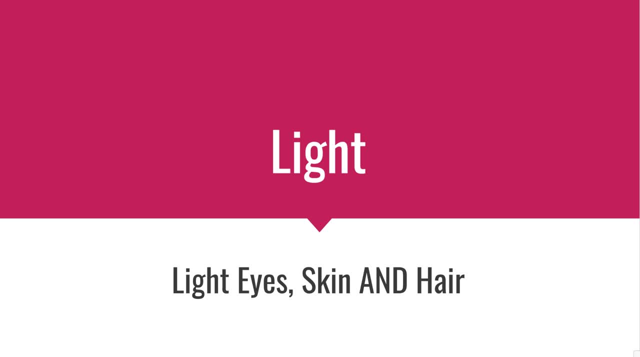 So we're going to use white and then you're going to choose your choice of brown. Now, the first part of your colored palette is going to be something like what you like to have in your. if you are light, it means you have light eyes, skin and hair- the whole combination of the three. 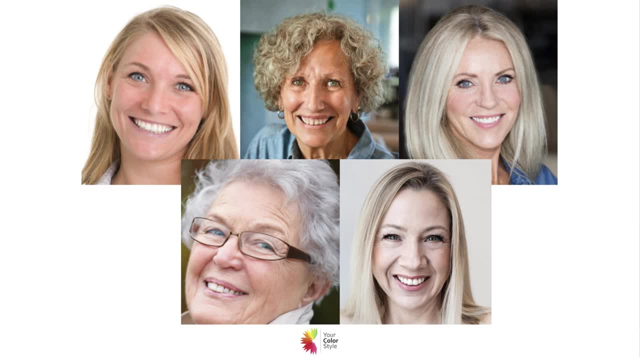 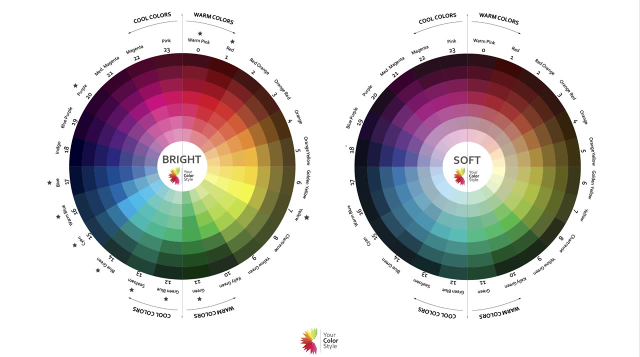 features needs to be light. if you have brown eyes, you are not light. if you have darker hair, you are not light, and if you have brown skin, you are not light. now, this is important because when you look at the color wheels- and these are the bright and soft color wheels with the full spectrum of color- 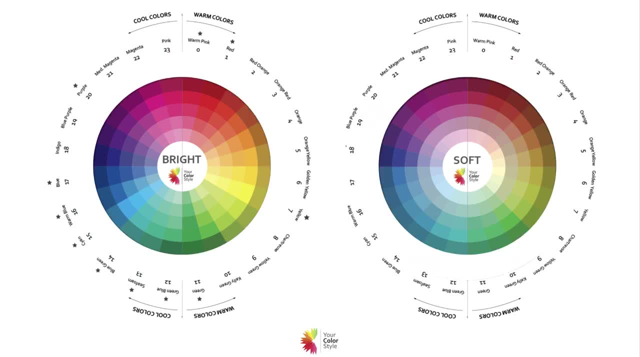 if you are light, the sweet spot for your color range is here. it's just a little bit darker than the brightest ring down to the lights. that's your sweet spot of color. going too dark might feel too heavy because your contrast is very low and we're looking for colors that are 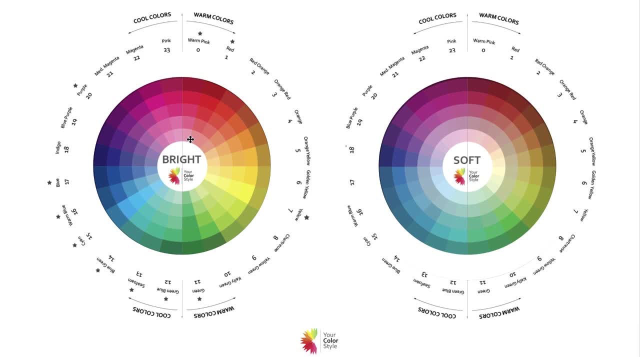 in harmony with you. so that's why it's important to know if you are light. if you have gray blend hair with some brown in it, you're probably more medium. if you have medium to dark brown hair that you've highlighted blonde, you are not light, okay, even though your hair is lighter. so you need 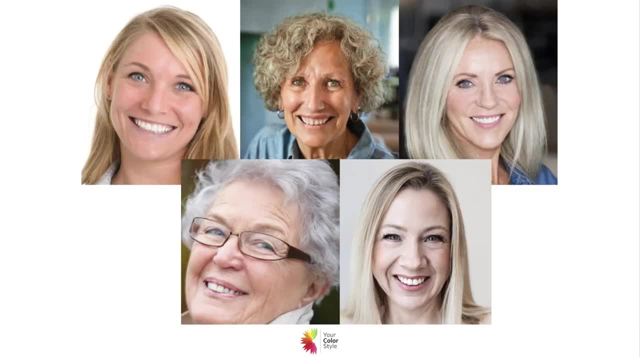 to have light eyes, skin and hair and that can be light blonde, golden, blonde, dark blonde, white hair, gray hair, silver hair, anything like that, and then the eyes would be blue, green, green, blue, light eyes. they can have a little other color, like blue, could have a touch of brown, but it needs to. 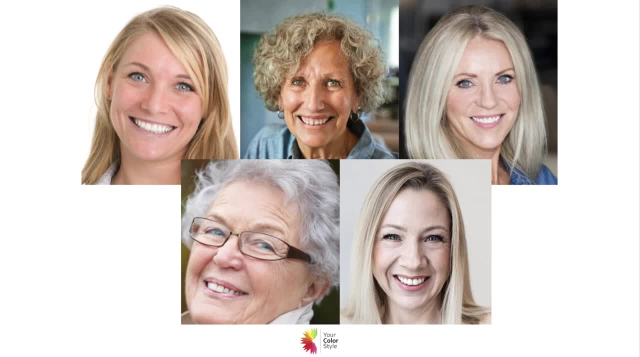 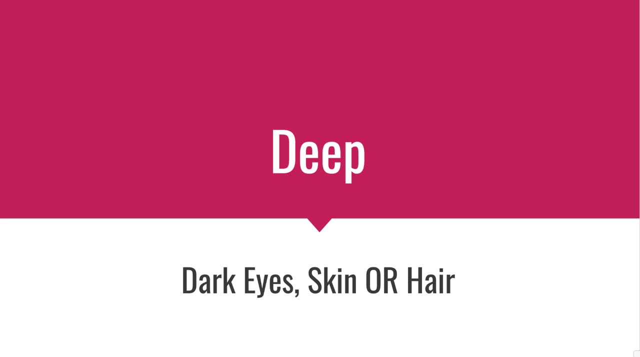 read like gray blue, that kind of a thing. so those are light eyes, light skin and hair. you are light. now there's deep. deep means you have dark eyes, dark skin or and dark hair. you need to have at least one of those three. the more you have of those. 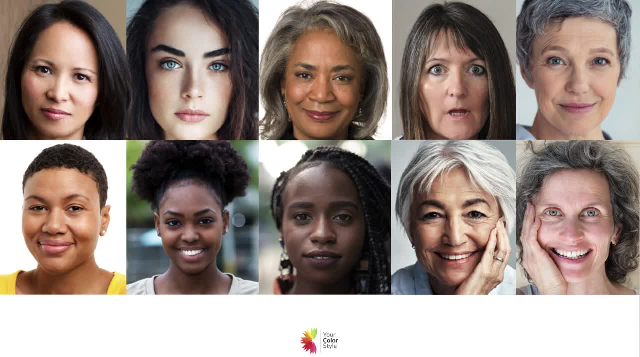 features. obviously, the more you can easily say you are deep. so notice, here you have a wide variety of individuals that are all considered deep. if you have salt and pepper hair with dark hair showing you are deep, okay, so notice. the two men on the right have salt and pepper and gray blend. 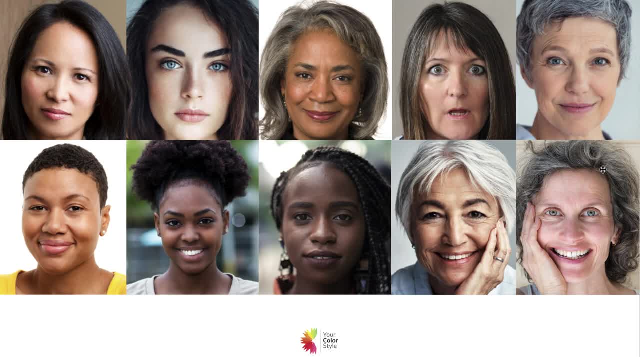 with dark hair in there. they were probably naturally dark at one time. I would put them in the deep category. okay, dark eyes, dark skin, dark hair- one of those, or all three, or just two, will make you deep, and that's important because when you look at the color wheel, 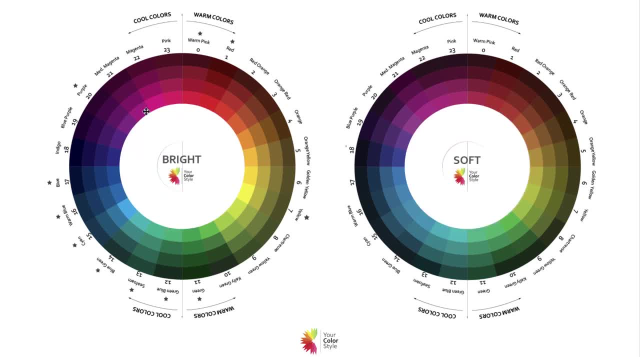 your sweet spot of color is the brightest ring to the darkest ring. now that doesn't mean that you can't wear colors that are lighter, but most of the color types that are deep don't look great in pastels. the only color type that looks really good in like icy pale colors, would be bright, cool and 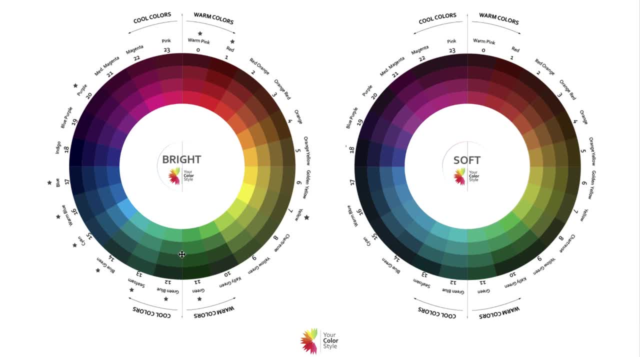 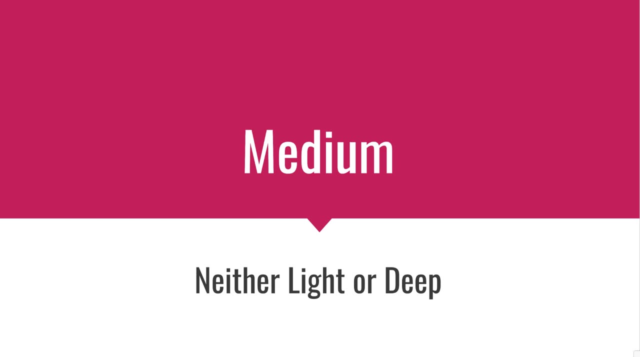 deep. okay, but this is your sweet spot of color. lighter colors might drain you and not be as flattering as these richer, deeper tones. and then we have medium. medium is: if you are not light and you are not deep, then you are medium. make it easy on yourself. 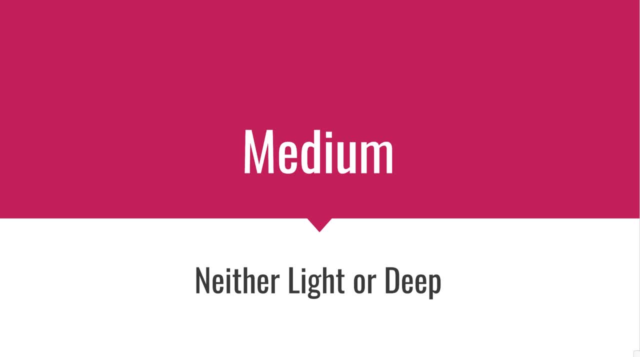 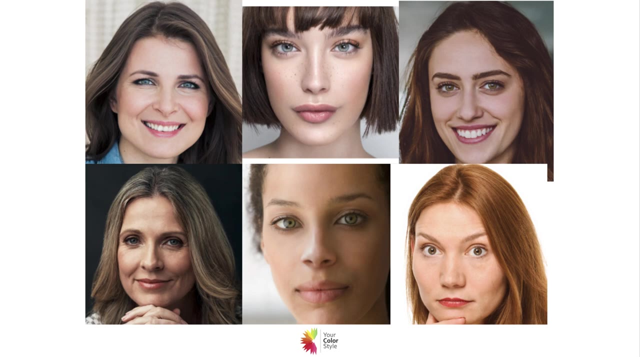 when you are light. if you feel like you're in between medium and deep, choose medium colocations for medium tones. just choose medium because you can always go darker. you are medium if you have medium brown hair, orange, Reed or black paint colors that are often darker than and medium. I would always choose medium because you are medium if you. 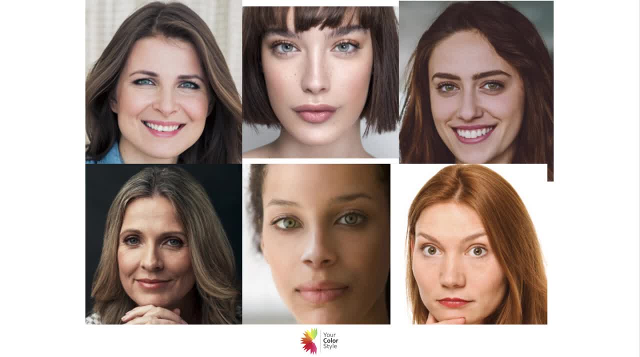 have a medium brown hair, MHла, mediumtimещ, sure. dark eyes, medium brown eyes, medium hazel eyes- all those as long as your darkest feature isn't darker than medium. If you have a very dark feature, you're going to fall in, probably more. 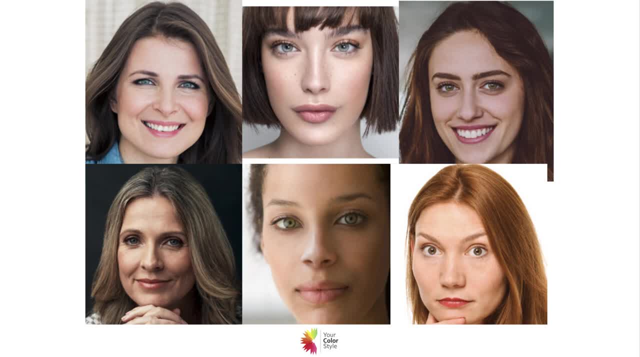 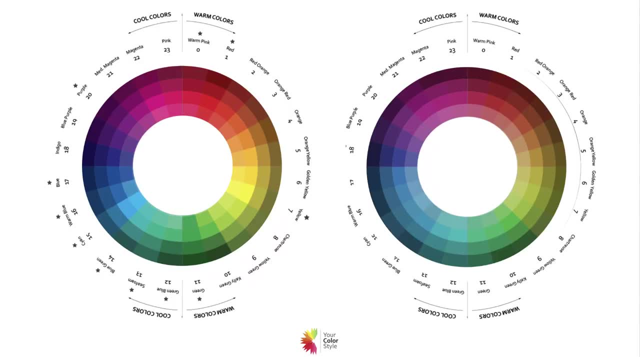 into the deep category. So if you don't know if you're medium or deep, it's always safe to choose medium, Because the difference here is that your sweet spot of color will be just a little bit lighter, not much than the bright ring here and then going darker. So if you decide that you 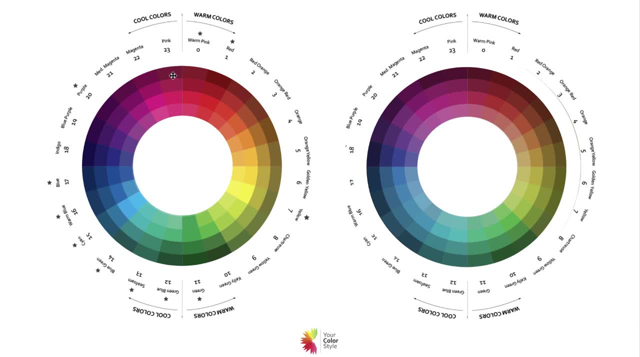 choose medium and then later realize that you could probably wear darker colors. you can, There's nothing that says you can't- And this flexibility here allows you to just simply go darker. And you don't necessarily need another color fan, unless you want one. You can just go darker. 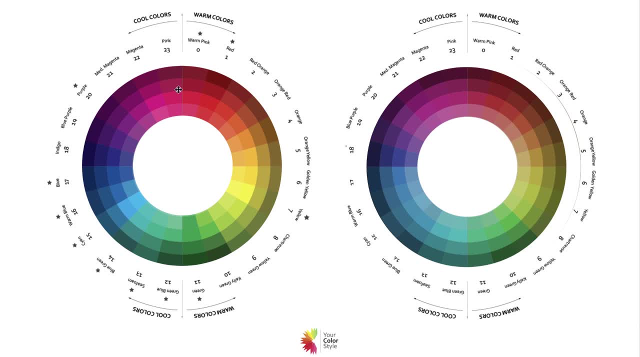 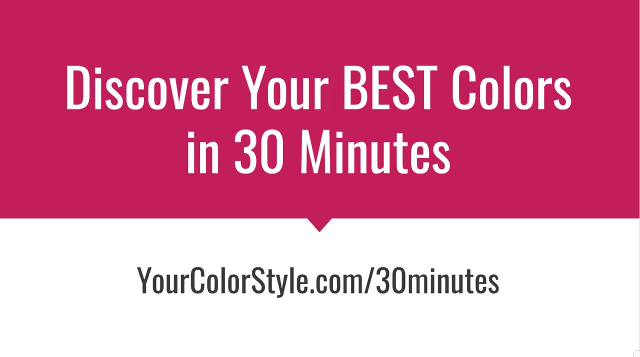 on the rings of color. Okay. so if you are not light or deep, choose medium. And now you have narrowed yourself down to, just now, four color types. So if you want a really fun, quick and easy way to learn your color type, especially after you've. 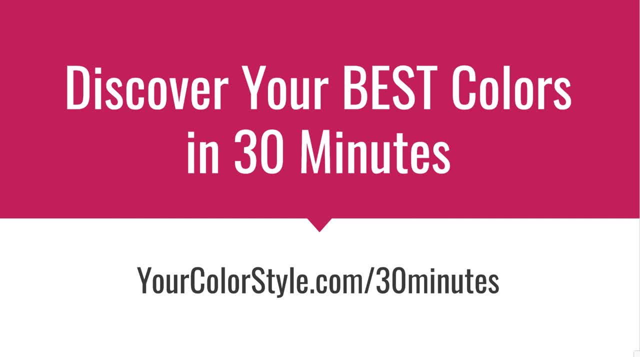 learned, whether you are light, medium or deep. take my webinar: Discover Your Best Colors in 30 Minutes. This webinar is designed to be quick: Only 30 minutes. You've got 30 minutes And at the end of this webinar, you will hopefully know your.